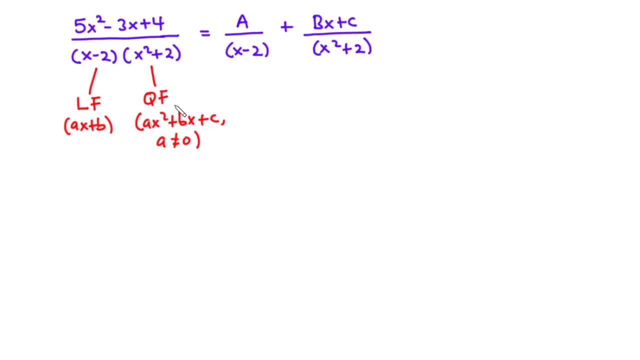 equal to 0. Now if the denominator of a rational function is made up of a linear factor and a quadratic factor, then decomposing this rational function into partial fractions, the numerator of the linear factor is a constant which is represented by a and the numerator of the quadratic factor is linear represented by bx plus c. So the numerator of the linear factor is a constant which is represented by a and the numerator of the quadratic factor is linear represented by bx plus c. So in other words, we can say that the numerator of each of the factors 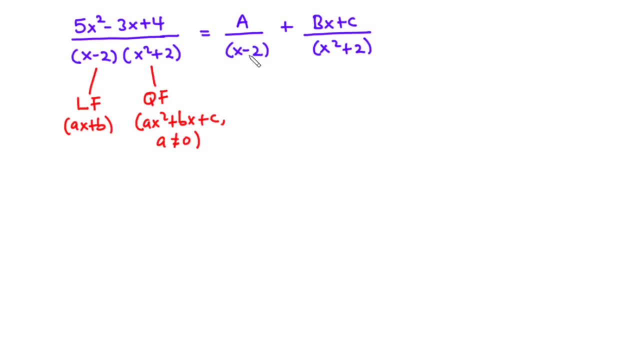 is 1 degree less than the denominator. The numerator of each of the factors is 1 degree less than the denominator. Now let's find the LCM and then work out this to find the values of a, b and then c. 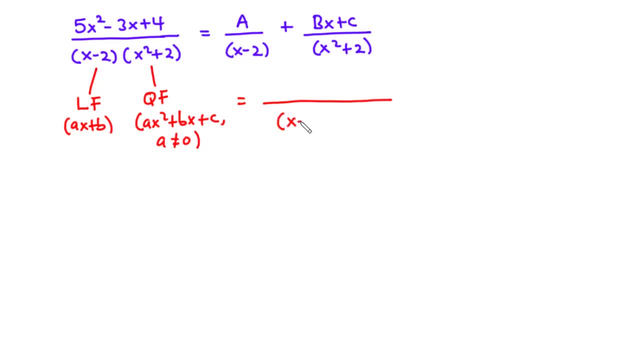 So the LCM becomes x minus 2 times x square plus 2. So we divide x minus 2, x square plus 2 by x minus 2 and then we are left with x square plus 2. So we have a times x square plus 2 plus, we divide x minus 2, x square plus 2 by x square plus 2 and then we have x minus 2 left. 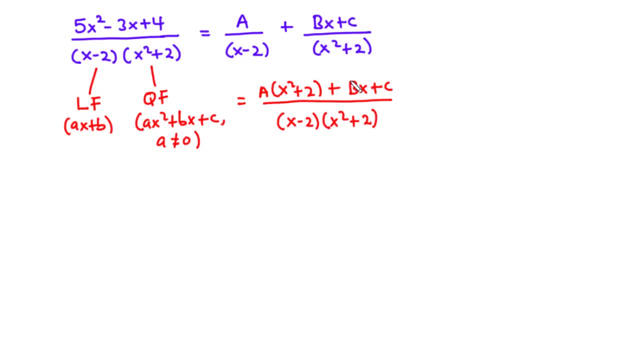 So that is bx plus c times x minus 2. 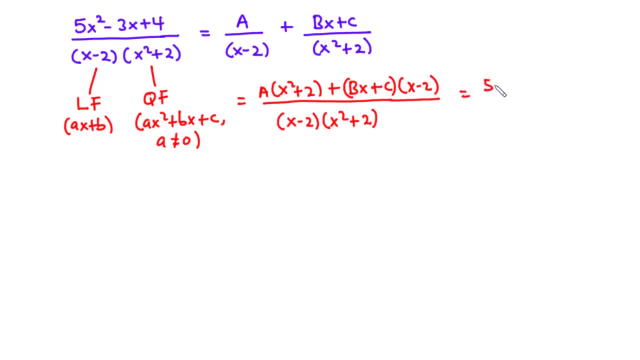 Now this is equal to the rational function 5x square minus 3x plus 4 divided by x minus 2, x square plus 2. Now since the denominator is the same we can compare the numerator and find the values of a, b and c. So this becomes a times x square plus 2 plus bx plus c times x minus 2 equals 5x square minus 3x plus 4. 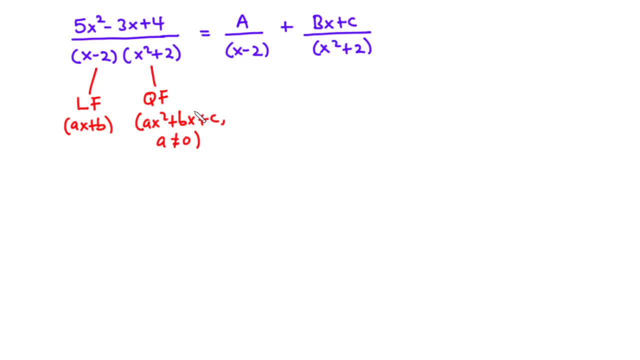 represented by bx plus c. So in other words, you can say that the numerator of each of the factors is one degree less than the denominator. The numerator of each of the factors is one degree less than the denominator. Now let's find the LCM. 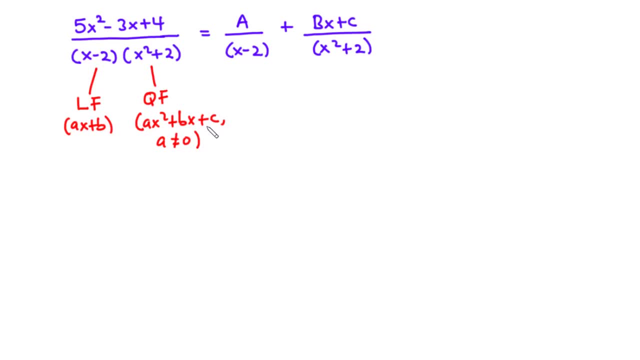 and then work out this to find the values of a, b and then c. So the LCM becomes x minus 2 times x squared plus 2.. So we divide x minus 2, x squared plus 2 by x minus 2. 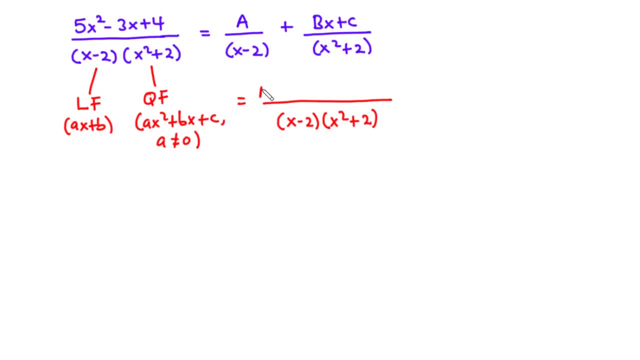 and then we are left with x squared plus 2.. So we have a times x squared plus 2, plus we divide x minus 2, x squared plus 2 by x squared plus 2, and then we have x minus 2 left. 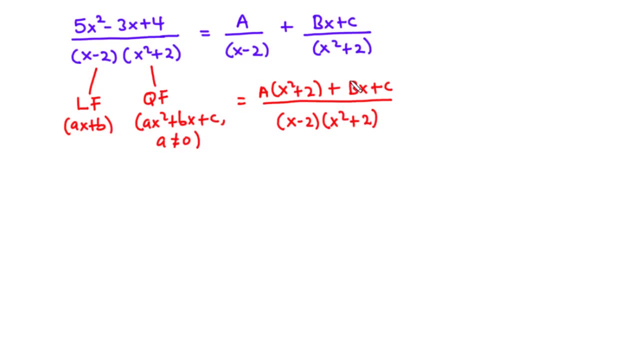 So that is bx plus c times x minus 2.. Now this is equal to the rational function: 5x squared minus 3x plus 4 divided by x squared plus 2 times x squared plus 2.. Now, since the denominator is the same, we can compare the numerator. 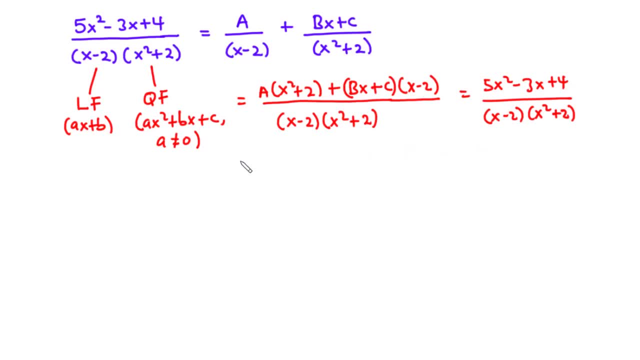 and find the values of a, b and c. So this becomes a times x squared plus 2 plus bx plus c times x minus 2 equals 5x squared minus x squared plus 2.. 3x plus 4.. Now we have x squared plus 2.. 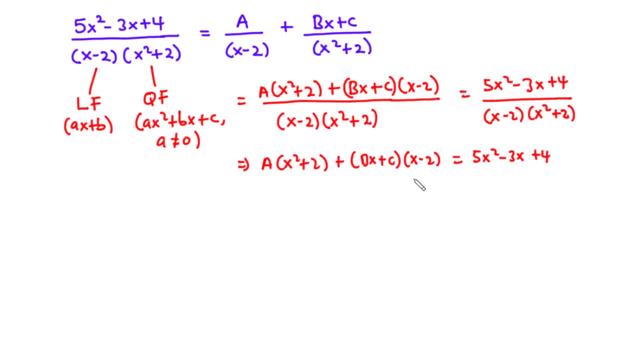 We have x minus 2.. So if we should put x equals 2,, then we have 2 minus 2, which is 0. Then we can do away with this term and then we focus on a and find the value of a. 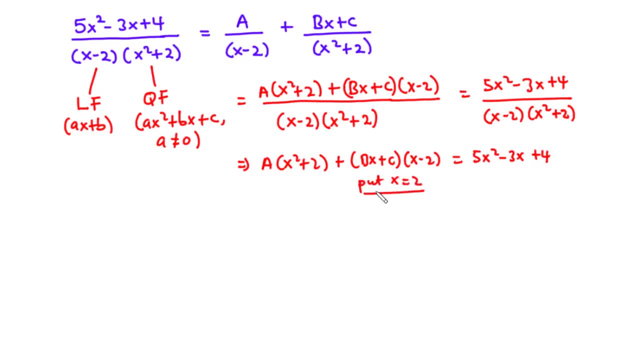 So let's put: x equals 2.. So we have a times 2 squared plus 2 plus bx plus c. b times 2 plus c. times 2 minus 2 equals 5 times 2 squared minus 3 times 2 plus 4.. 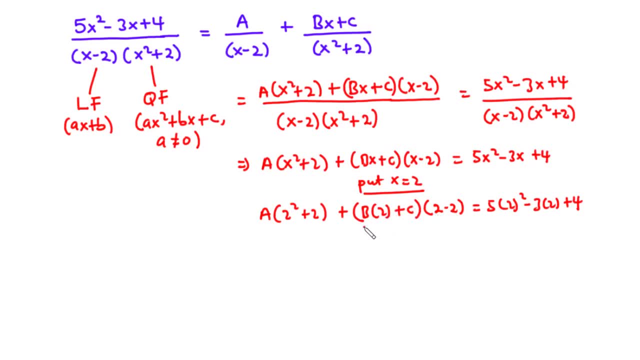 2 minus 2 is 0.. 0 times anything here is still 0.. 2 squared is 4 plus 2 is 6.. So we have 6a equals: 2 squared is 4 times 5 is 20.. 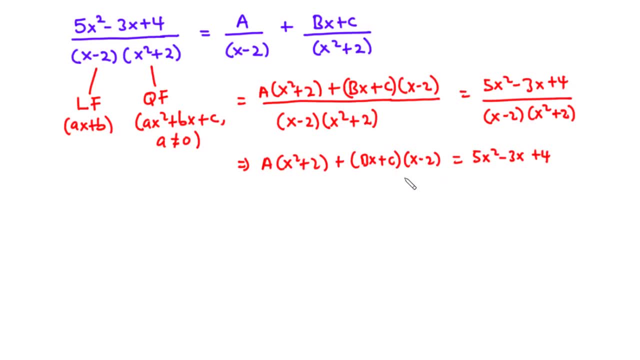 Now we have x square plus 2 we have x minus 2. So if we should put x equals 2 then we have 2 minus 2 which is 0. Then we can do away with this term and then we focus on a and find the value of a. 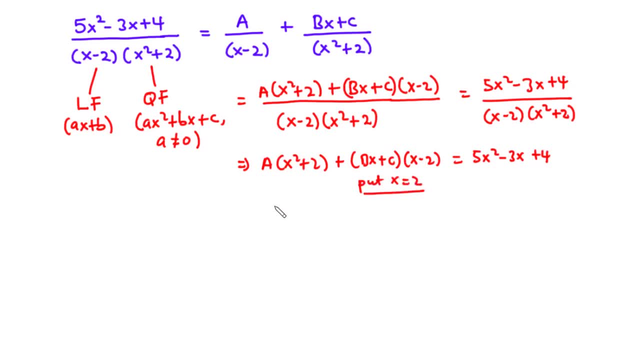 So let's put x equals 2. So we have a times 2 square plus 2 plus 2x. 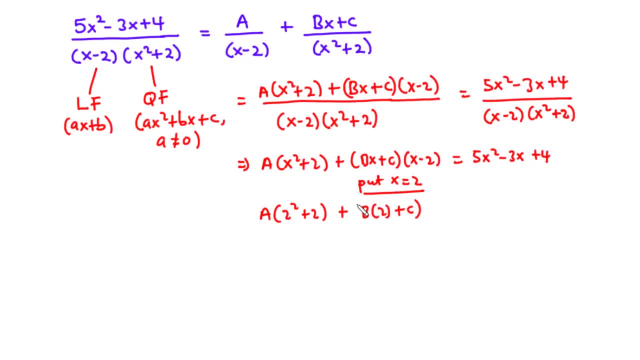 b times 2 plus c times 2 minus 2 equals 5 times 2 squared minus 3 times 2 plus 4. 2 minus 2 is 0. 0 times anything here is still 0. 2 squared is 4 plus 2 is 6. 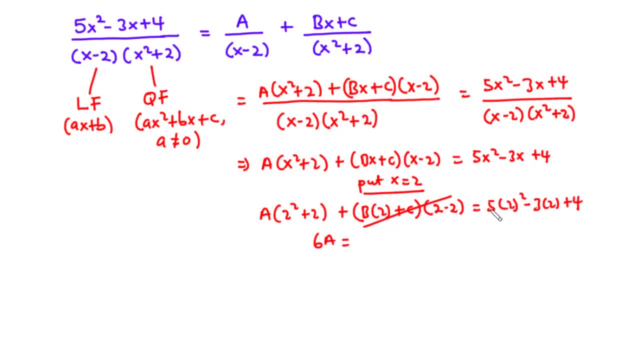 So we have 6a equals 2 squared is 4 times 5 is 20. 20 minus 6, we have 14. 14 plus 4 is 18. 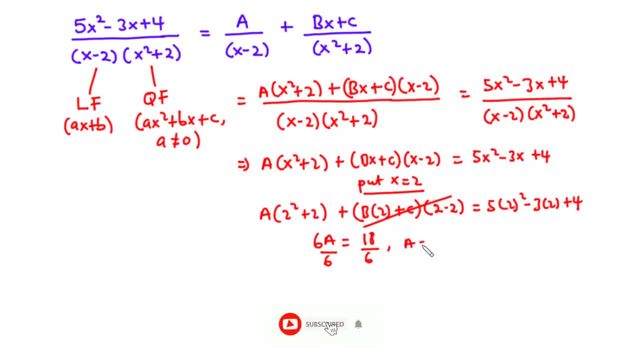 You divide 3 by 6, we have the value of a to be thrown. So this is a. 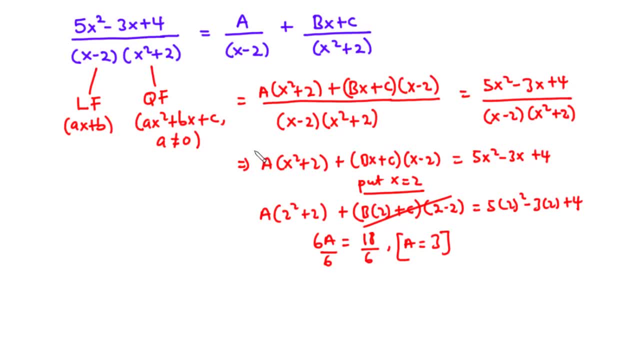 Now let's find the value of b and then c. To find the value of b and c, we need to expand this identity. So we have a times x squared, that is ax squared, plus a times... times 2 is 2a. 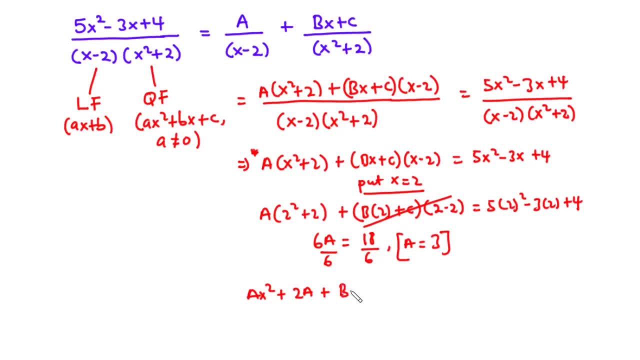 Plus we have bx times x, that is bx squared. c times x is... We have cx. 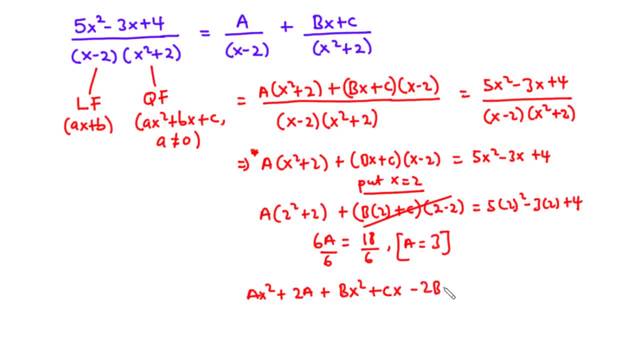 bx times negative 2, we have negative 2bx. And then c times negative 2 is negative 2c. 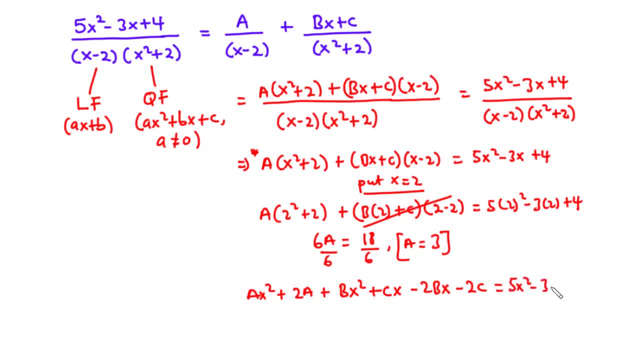 This is equal to 5x squared minus 3x plus 4. 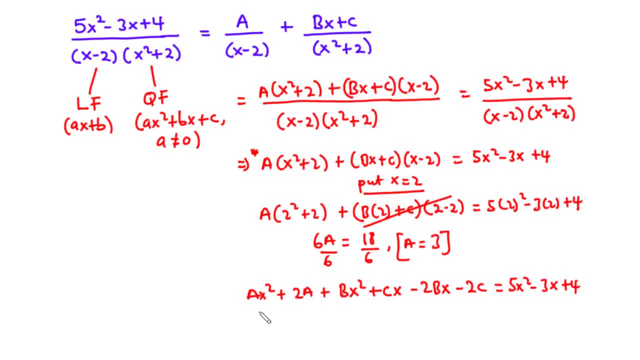 Now let's group like terms and factor. Let's put out the common term. 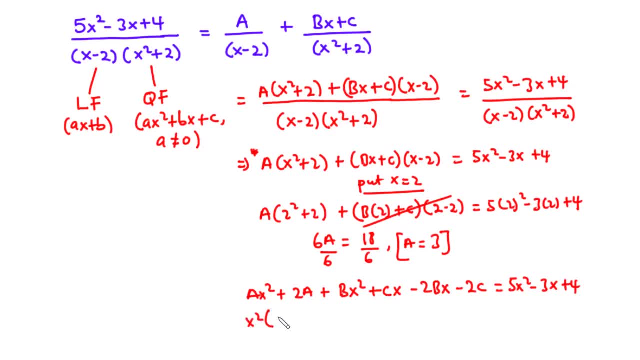 So for x squared, we have x squared outside and then a plus b. 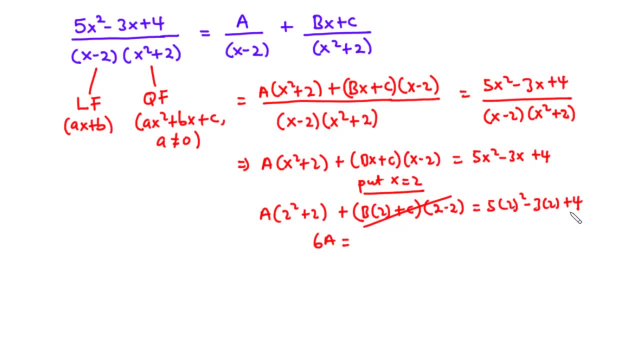 20 minus 6, we have 14.. 14 plus 4 is 18.. You divide 3 by 6. We have the value of a to be throwing. So this is a. Now let's find the value of b and then c. 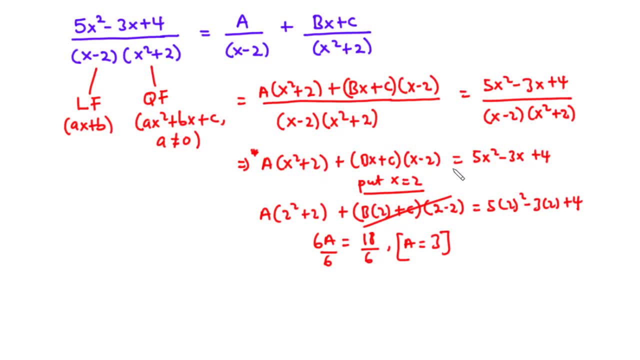 To find the value of b and c, we need to expand this identity. So we have a times x squared, that is ax squared, plus a times 2 is 2a. So we have a times x squared that is: ax squared plus a times 2 is 2a. 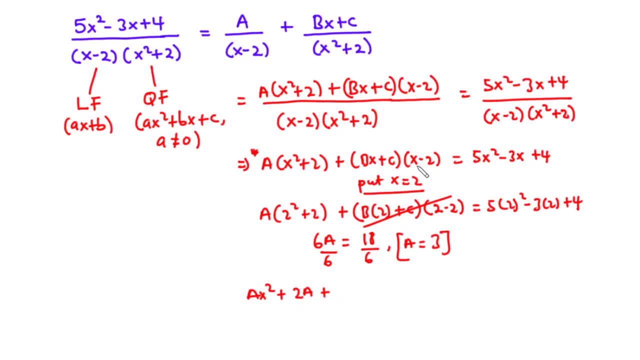 plus we have bx times x, that is bx square. c times x is we have cx. bx times negative 2. we have negative 2 bx and then c times negative 2 is negative 2c. this is equal to 5x square minus 3x. 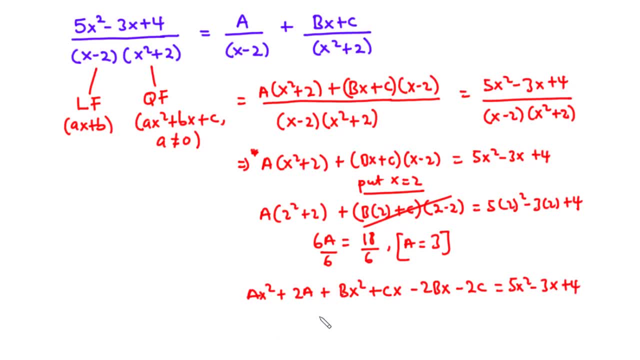 plus 4. now let's group like terms and factor out the common term. so for x square we have x square outside, and then a plus b. for x we have x outside, and then we have negative 2b plus c, so negative 2b plus c, and then for the constants we have 2a minus 2c. 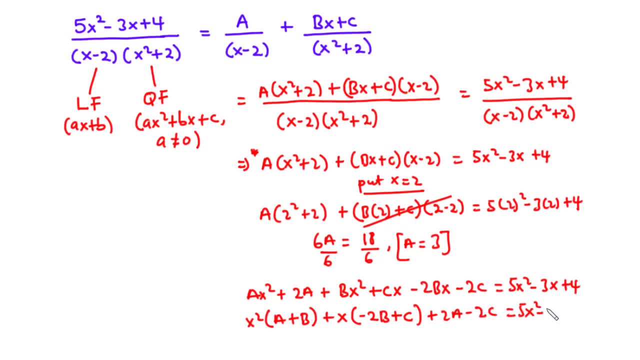 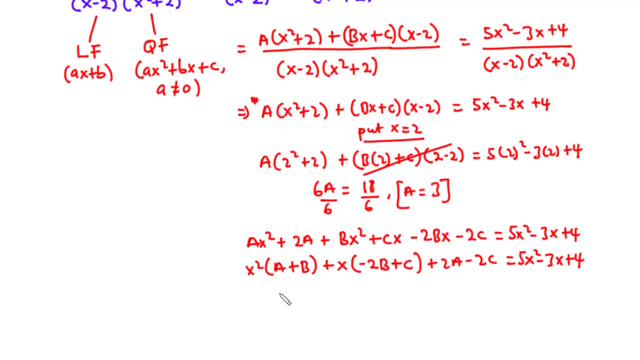 this is equal to 5x plus 4. now let's group like terms and factor out the common term equal to 5x squared minus 3x plus 4.. Now let's compare the coefficients of x squared. So compare coefficients of x squared. The reason why we are going to compare the coefficients of x squared is: 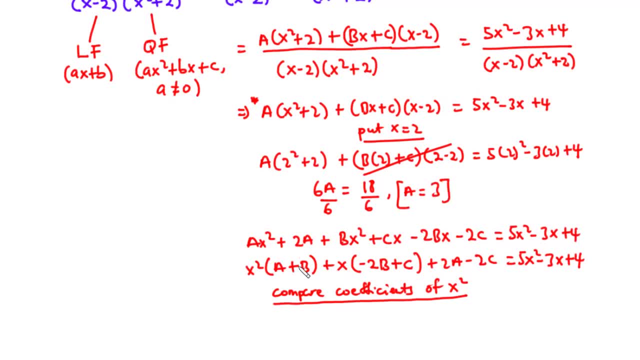 that we know the value of a to be 3, and then here we have a plus b. So if a plus b is equal to 5, then we can find the value of b. So a plus b is equal to 5.. We have a to be 3.. So right away we 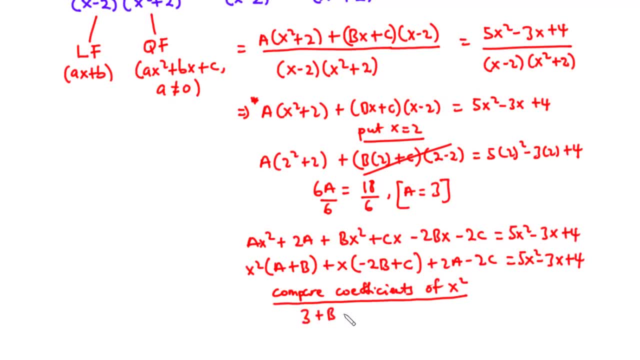 can write our 3.. So 3 plus b is equal to 5.. We transpose 3 to the right hand side. We have b equals 5 minus 3, which is equal to 2x squared. So we have a to be 3.. So we have a to be 3.. So we. 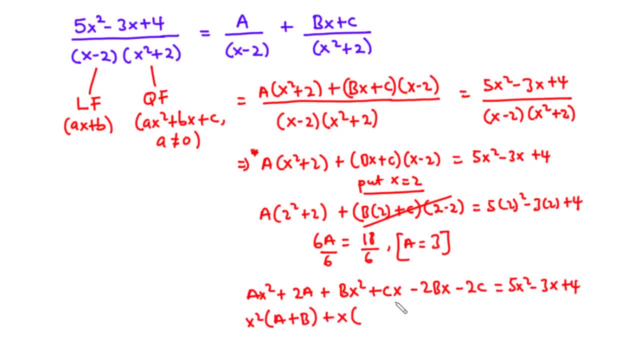 For x, we have x outside and then we have negative 2b plus c. 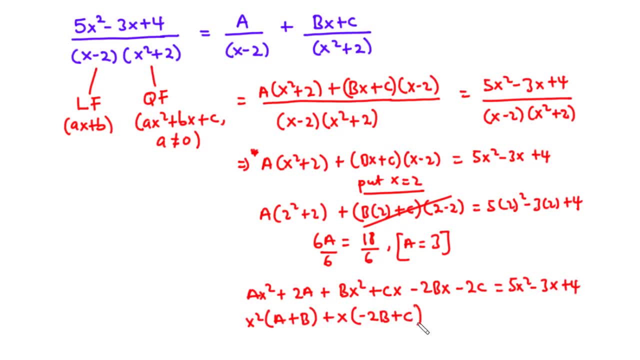 So negative 2b plus c. 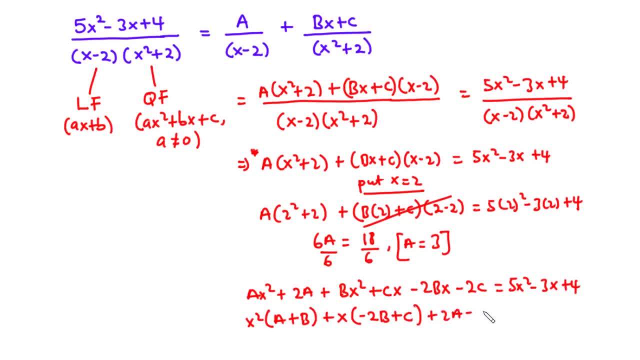 And then for the constants, we have 2a minus 2c. 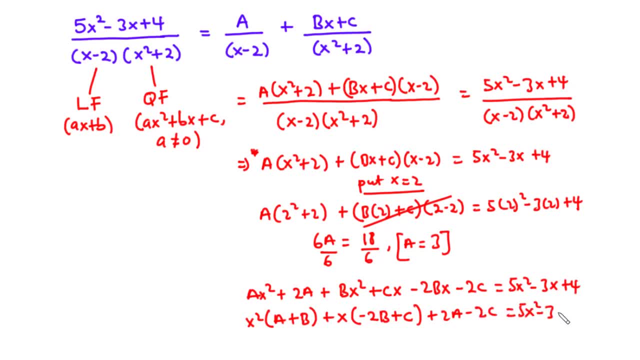 This is equal to 5x squared minus 3x. Plus 4. 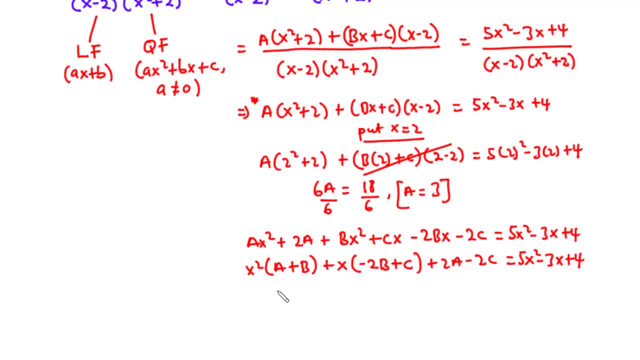 Now let's compare the coefficients of x squared. So compare coefficients of x squared. The reason why we are going to compare the coefficients of x squared is that we know the value of a to be 3 and then here we have a plus b. 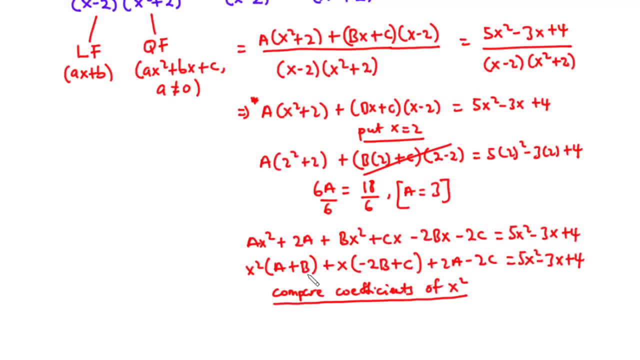 So if a plus b is equal to 5, then we can find the value of b. So a plus b is equal to 5. We have a to be 3. So right away, we can write our 3. So 3 plus b is equal to 5. We transpose 3 to the right hand side. We have b equals 5 minus 3, which is equal to 2. Therefore, the value of b is equal to 2. Now let's find the value of c. Since we have negative b plus c. 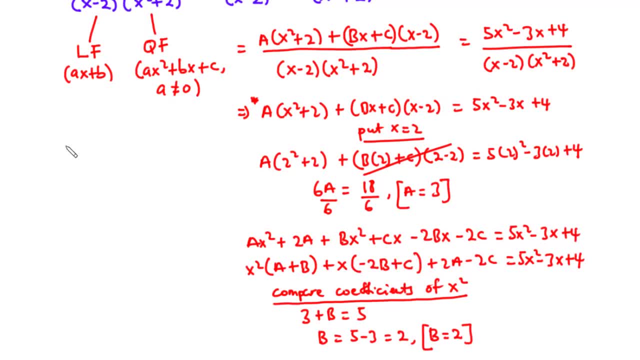 We can compare coefficients of x. So compare coefficients of x. 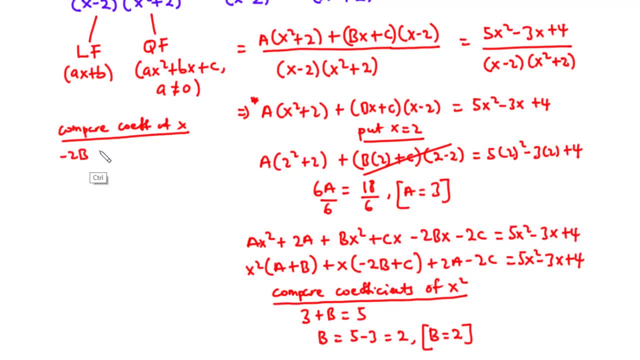 So negative 2b. We have b to be 2. 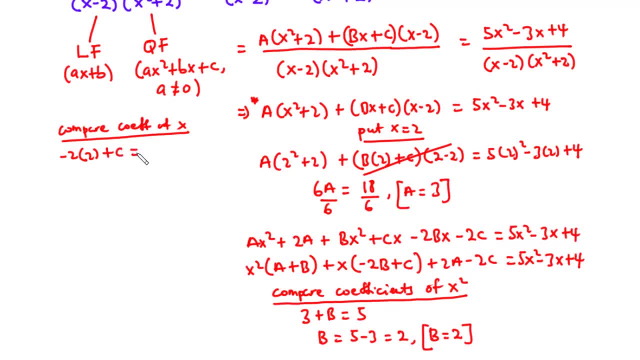 So negative 2 times 2 plus c is equal to negative 3. We transpose negative 2 times 2 to the right hand side. So we have c equals negative 3 plus 2 times 2. 2 times 2 is 4. 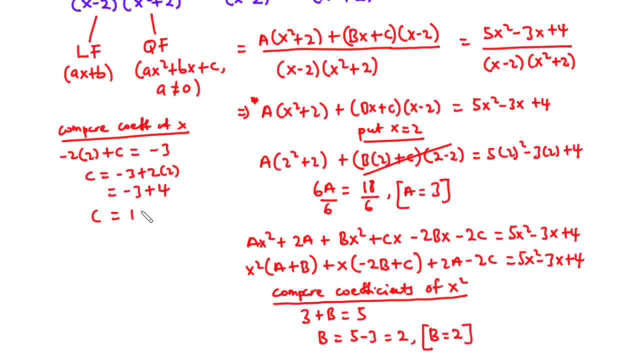 So we have c to be equal to 1. So a is equal to 3. b is equal to 2. And then c is equal to 1.